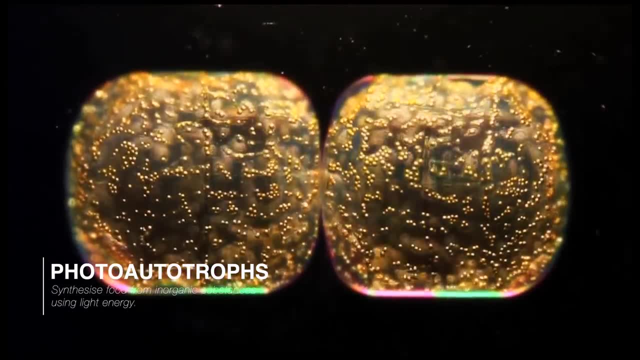 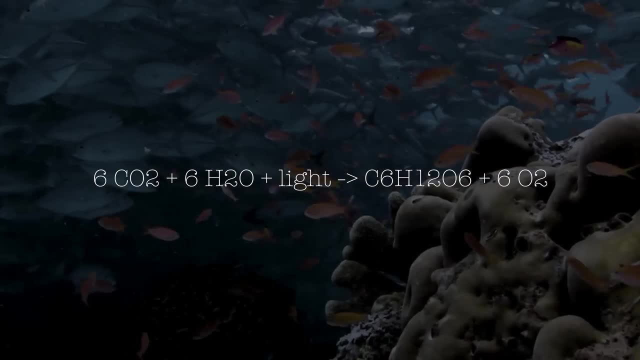 The photoautotrophs, Photosynthesising organisms that use energy from sunlight to convert carbon dioxide into oxygen and chemical energy stored as glucose. Though they are tiny, these plankton play a large role in the development of the food web. The food web of the deep sea is 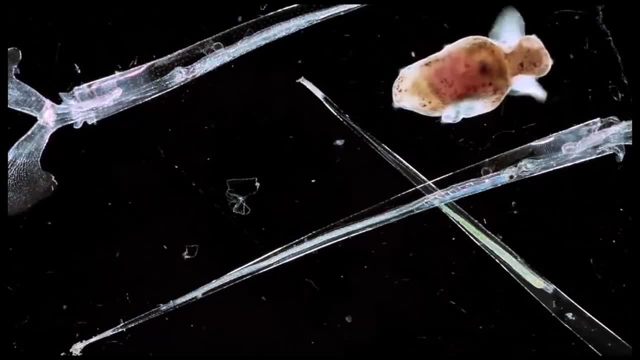 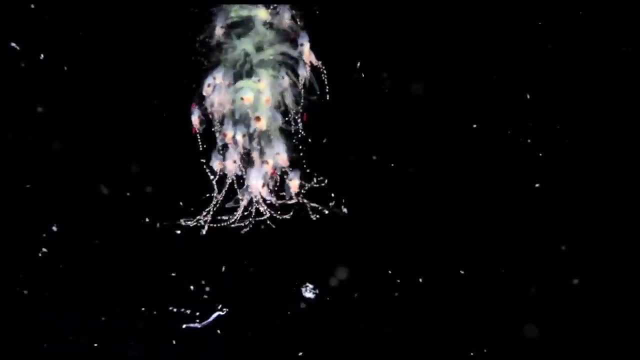 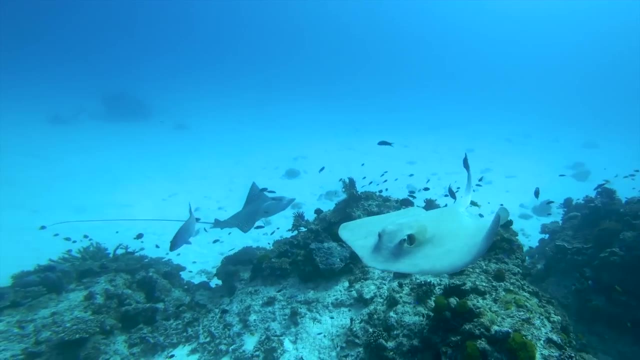 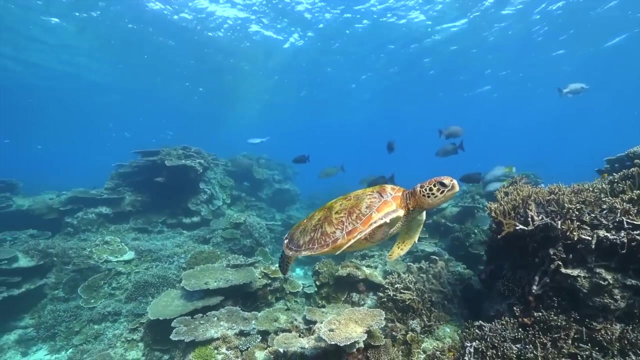 a large role, producing the carbon that supports nearly all marine life, as well as producing 50% of Earth's oxygen. Herbivores or primary consumers, such as zooplankton or turtles and manatees, feed primarily on the plants and phytoplankton. They assimilate what's left of the chemical. 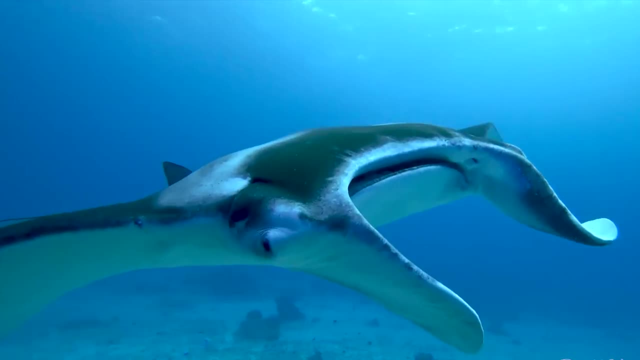 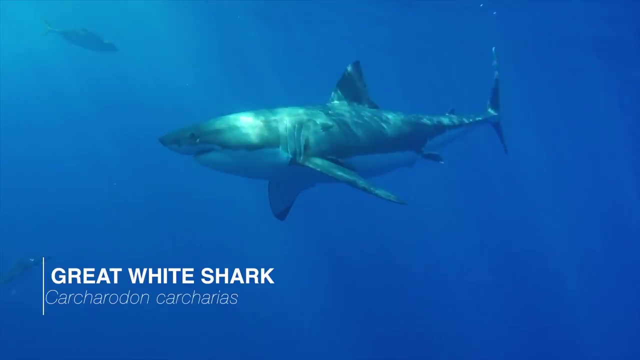 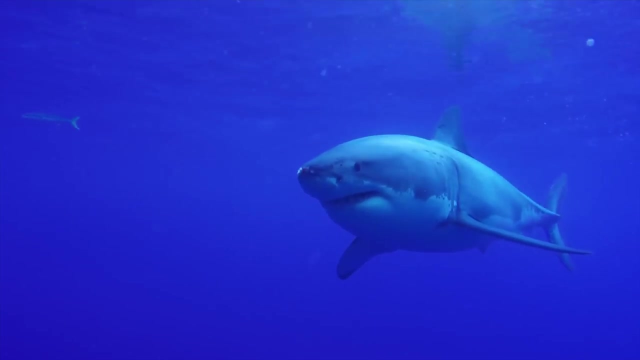 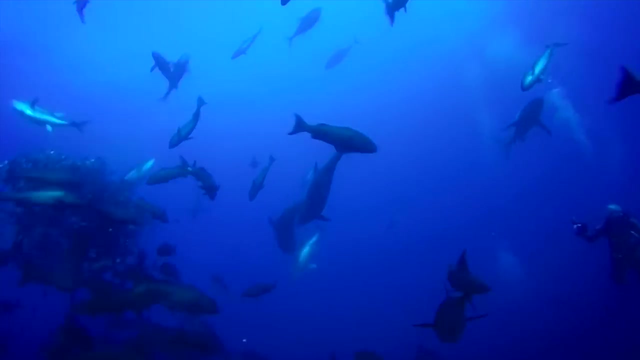 energy, using it themselves to grow and move. The herbivores become food themselves for secondary consumers, which make up the top two levels of the food web – carnivores and top predators. But amidst the productive frenzy of the shallow open ocean, animals excrete and die and molt. 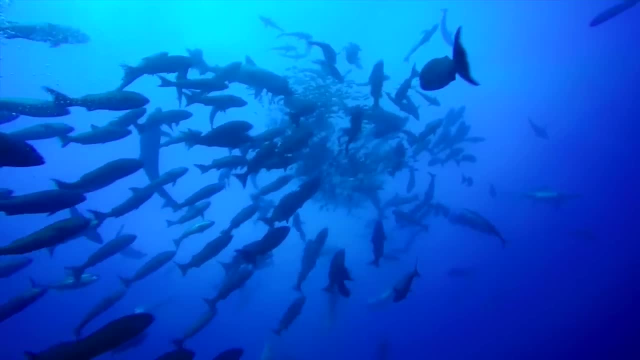 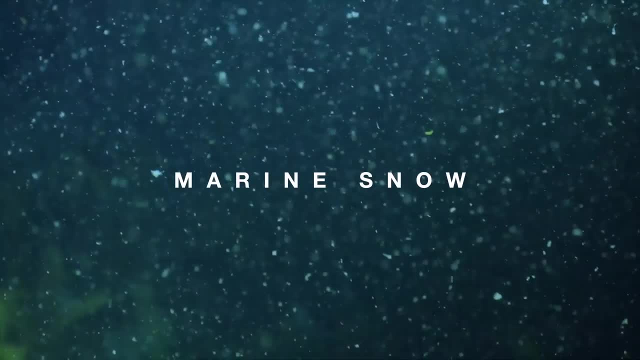 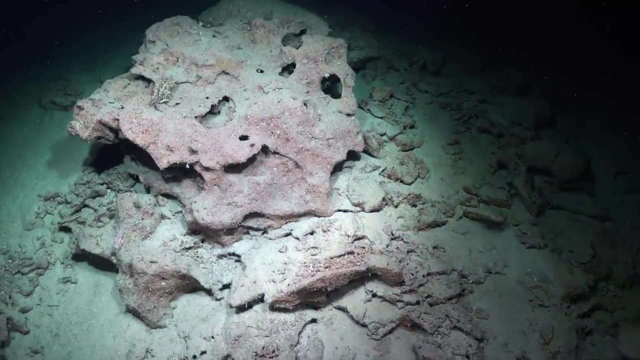 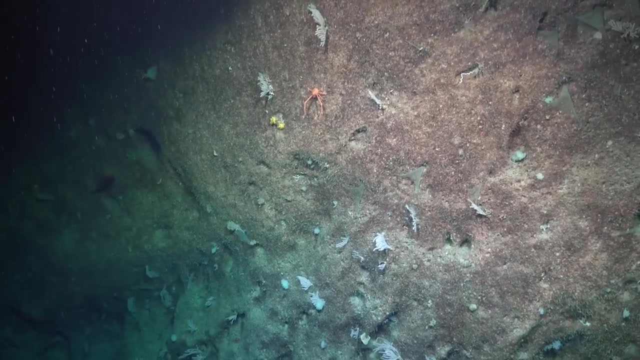 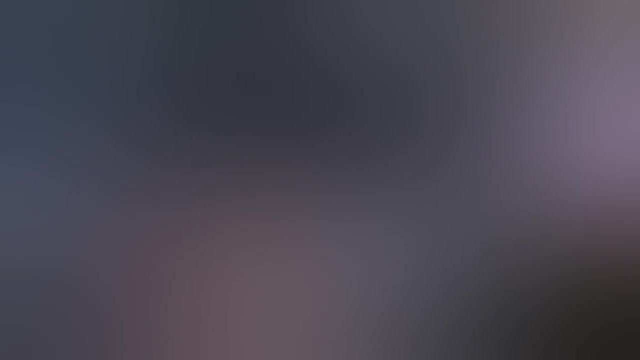 source of the food web. The food web is known as marine snow, And so we enter the isolated deep With no sunlight. photosynthesis cannot occur below 200 metres in the twilight zone. There are no plants here to fulfil the role of nutrient producers, There is only marine snow bringing. 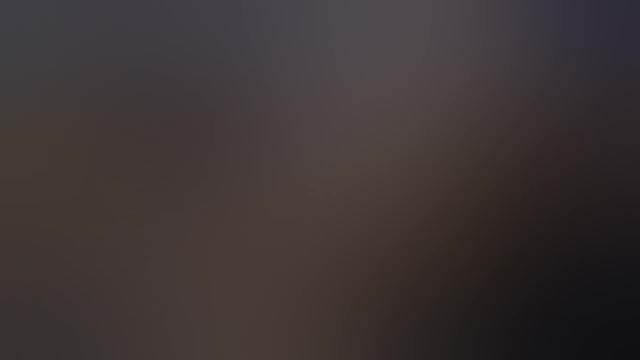 down the leftovers from above. It might be enough to sustain an abundance of food, but it's not enough to sustain an abundance of food. There is only marine snow bringing down the leftovers from above. It might be enough to sustain an abundance of food, but it's not enough to sustain an 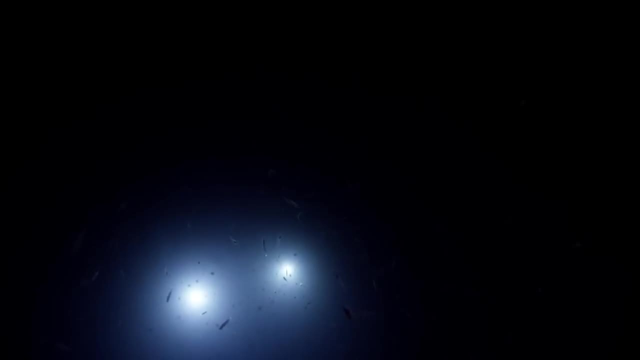 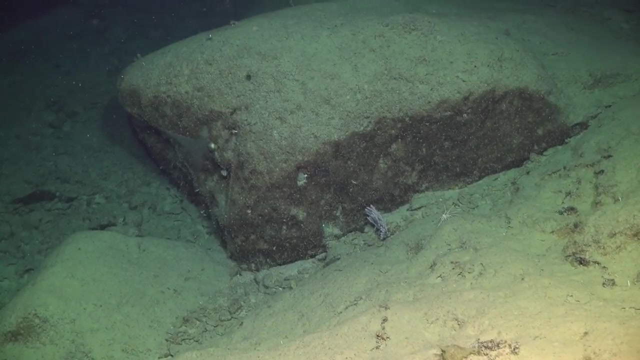 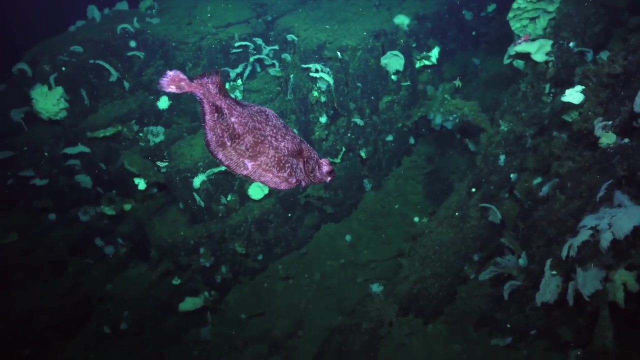 abundance of nutrients. There is only marine snow bringing down the leftovers from above. It might be enough to sustain an abundance of nutrients. There is only marine snow bringing down the leftovers from above. It's only a final change. So if the energy is not coming from the sun, then where is it coming from? 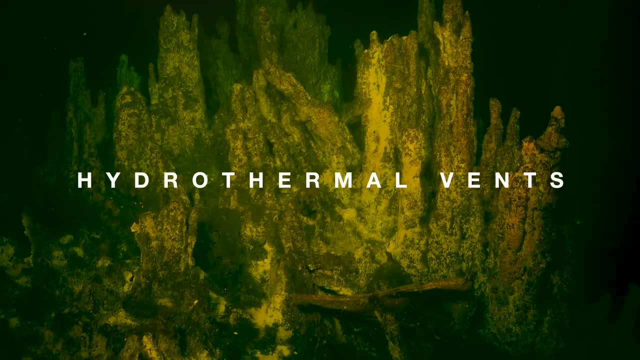 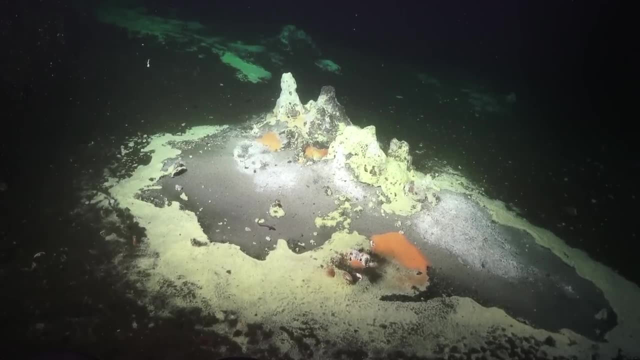 These are hydrothermal vents. It is just a hot up welling of dissolved chemicals and minerals that form towering chimney struckซ. these are hydrothermal vents. It is just a hot up welling of dissolved chemicals and chimney structures on the sea floor and release heated minerals from deep within the earth. 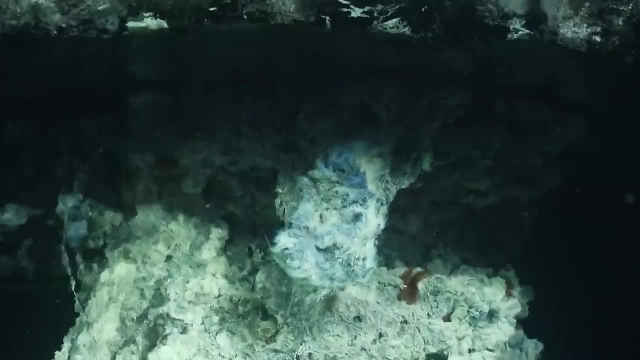 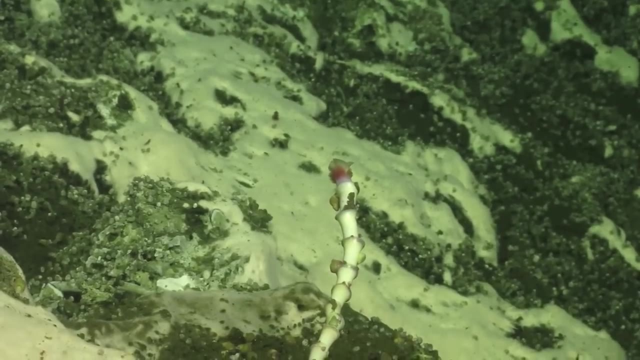 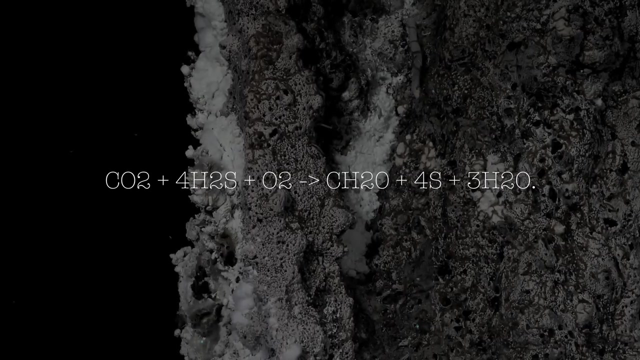 into the ocean. The chemicals expelled within the superheated vent fluid would be toxic to us humans, but to the life here they are vital, containing nutrients that bacteria are able to convert to energy in a process that mirrors the conversion of sunlight during photosynthesis. 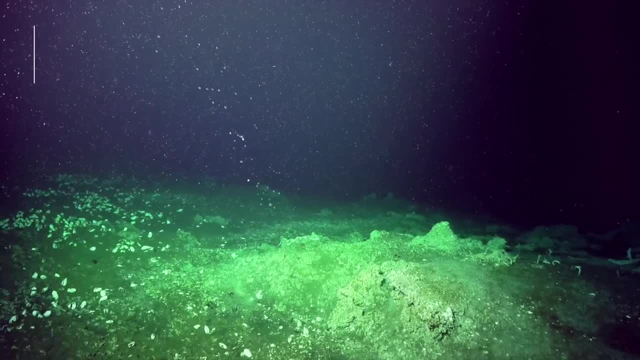 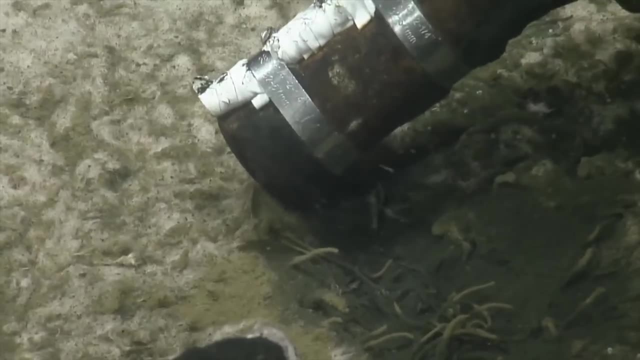 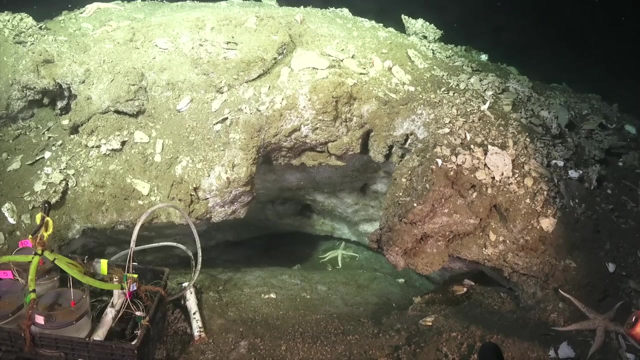 In place of photoautotrophs. we find chemoautotrophs. In place of plants and plankton, there is bacteria In place of photosynthesis, chemosynthesis. The bacteria are the primary producers, a major source of nutrients for the deep sea. 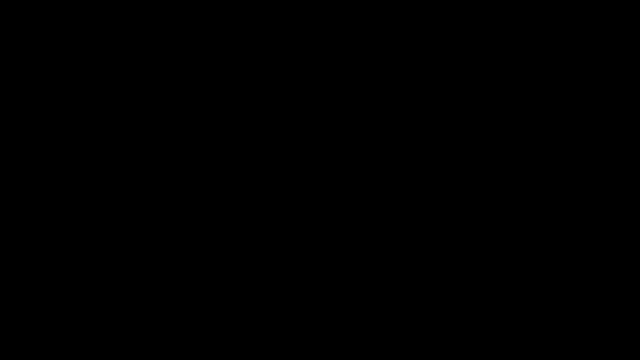 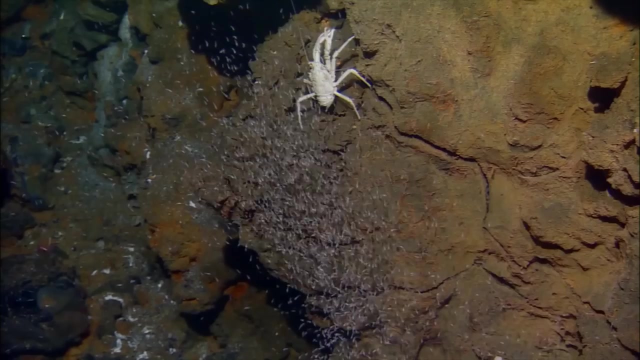 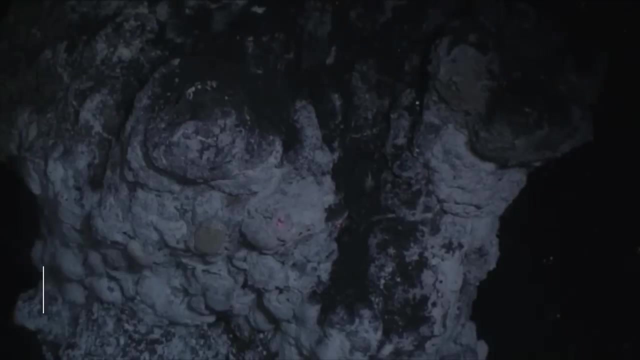 ecosystem. Like manatees grazing seagrass in the shallows, there are grazers here too. Bottom feeders like limpets and shrimps graze on the microbial mats. Yeti crabs farm colonies of the bacteria on their legs as a source of food. 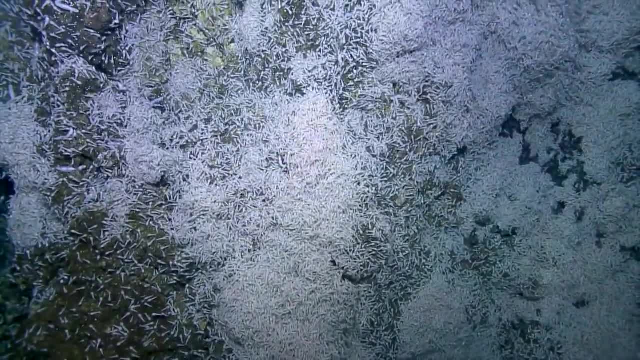 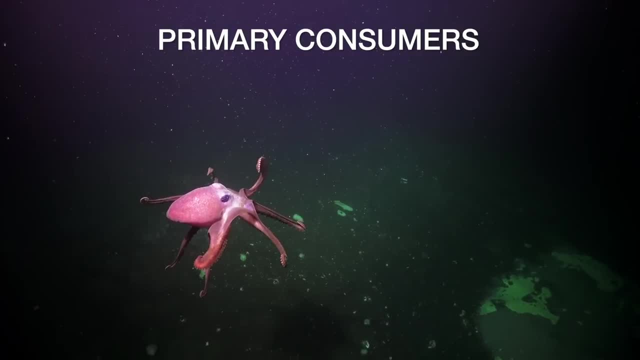 These creatures that rely on the bacteria for food are the deep ocean's primary consumers. Predators at the vents, such as crabs, eels and octopuses, are the secondary consumers. But here is where things get interesting. The deep ocean is a place of life. 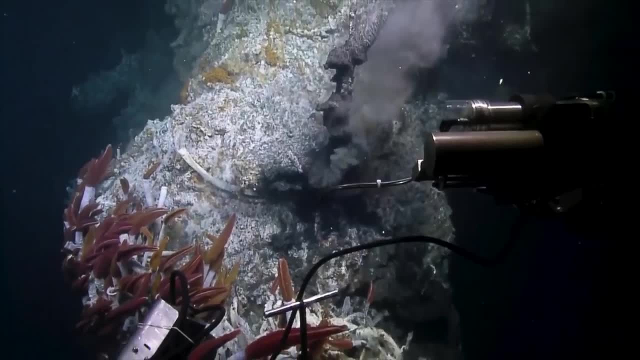 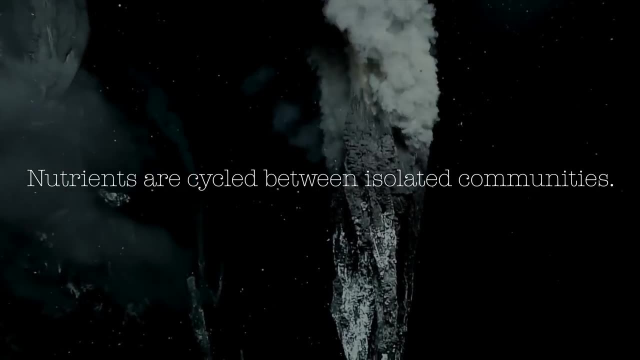 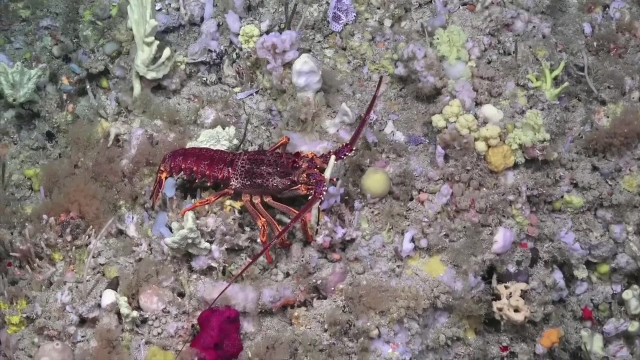 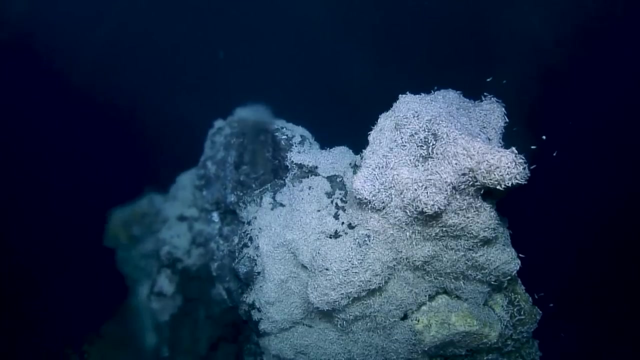 Though organisms at these isolated vent ecosystems cannot stray from their respective habitats, nutrients are still cycled between communities. The creatures here are demersal, meaning they live on or near the seafloor. They may be confined here, relying on the bacteria and unable to survive away from the 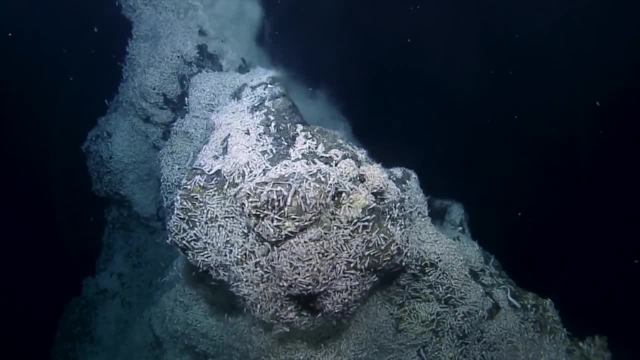 vent ecosystem, But a number of other processes contribute to the transformation of the ecosystem. For example, in the deep ocean there are many species that live on or near the seafloor. They may be confined here, relying on the bacteria and unable to survive away from the vent. 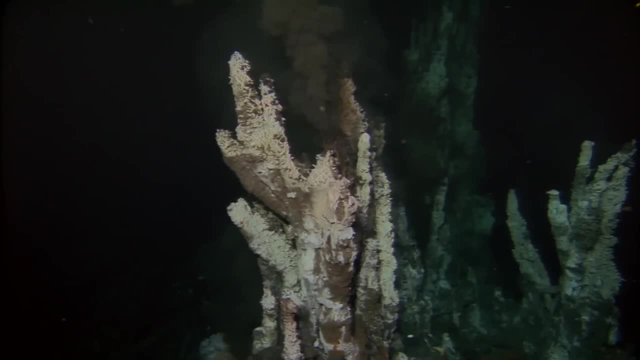 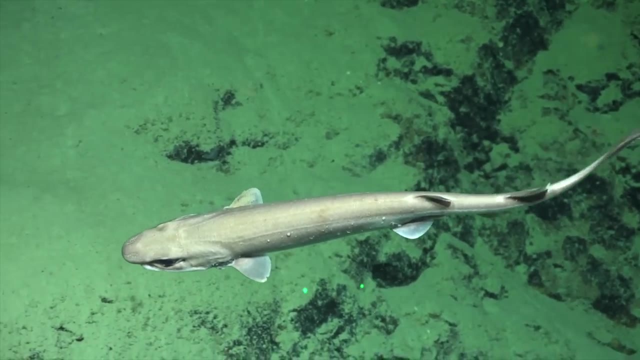 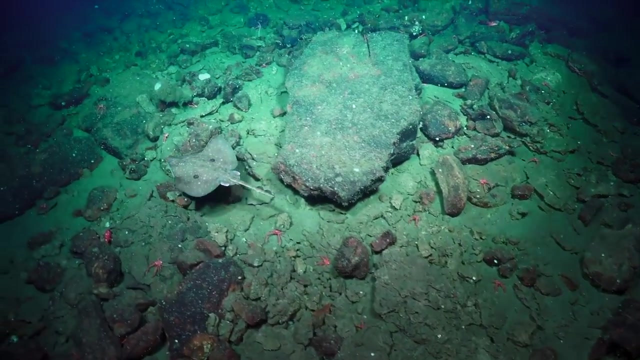 ecosystem. The first of these processes involves visitors to the vents. From hagfish to deep-sea skates, these are creatures that can survive away from the vents, but must seek out these hotspots of life in order to feed or lay their eggs. When they depart, they take any energy that they have assimilated with them and form a kind of supply chain. This means that they can survive on or near the seafloor, Moving energy from the source to the open ocean where there are no producers. 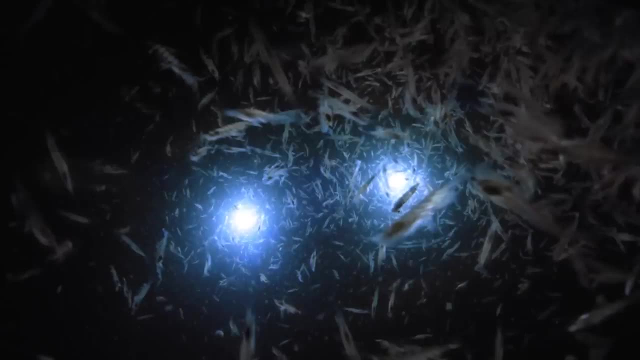 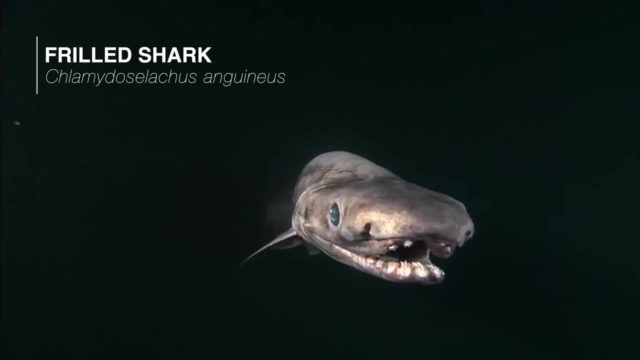 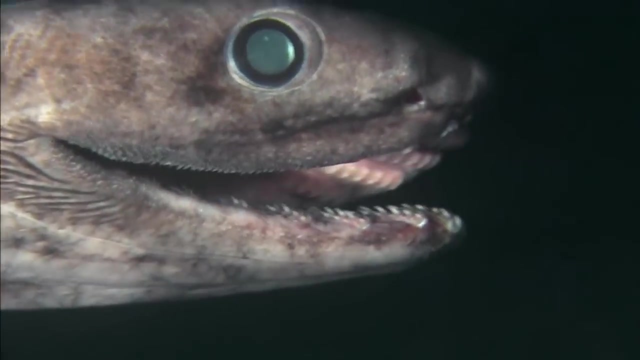 In doing so, these creatures are supporting another form of life in the deep sea, The pelagic ocean wanderers, ever moving and never settling as part of any one community. They get their energy through predation, feeding on the hagfish, skates and other organisms. 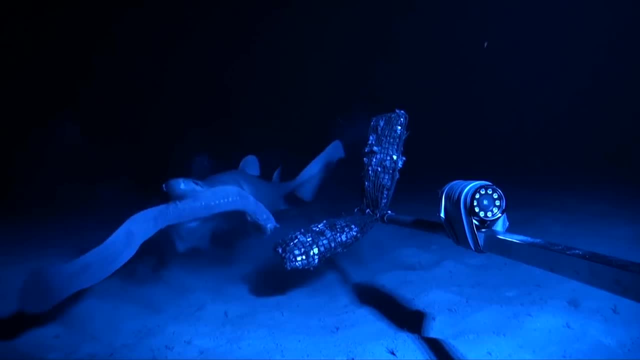 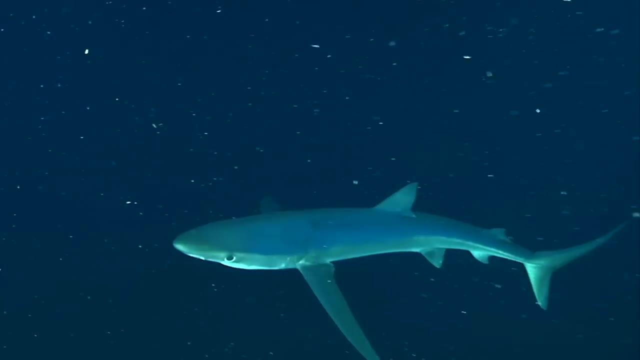 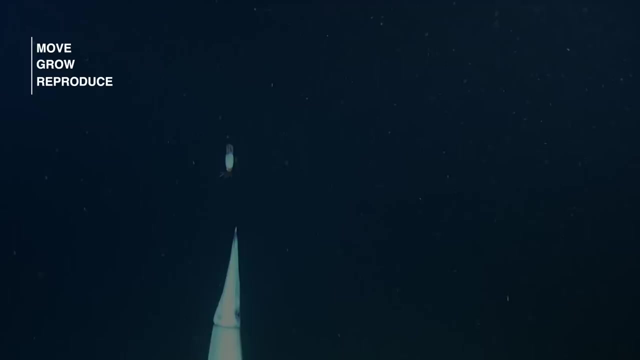 This means that they can survive on or near the seafloor. This means that they can survive on or near the seafloor. Energy is lost during its transfer from the vents to the open ocean. It is used up by the creatures as they move, grow and reproduce. so only a fraction of 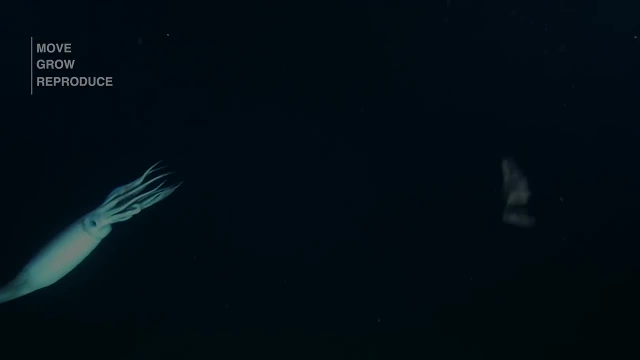 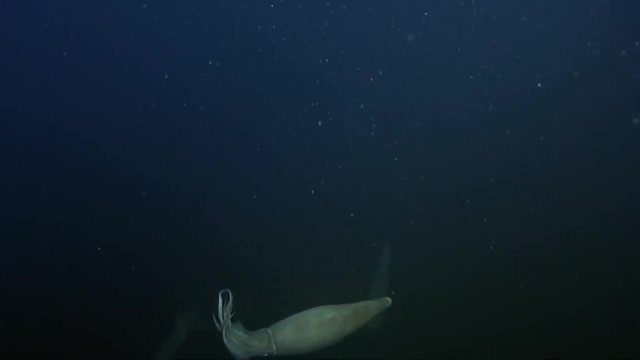 the nutrients they assimilate will make it to their predators. Thus, wanderers like the Humboldt squid tend to be larger, as they must be in order to become more efficient. This is because, although nutrients from vents and seeps are brought to them, they are far 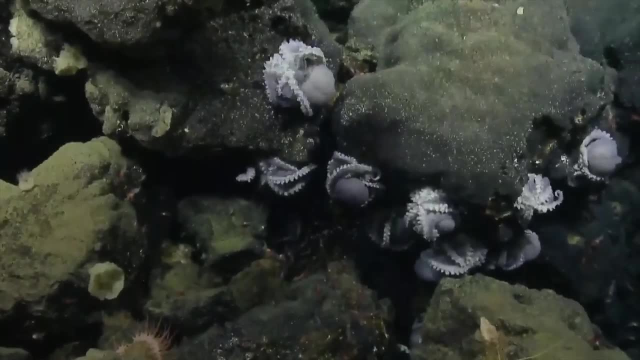 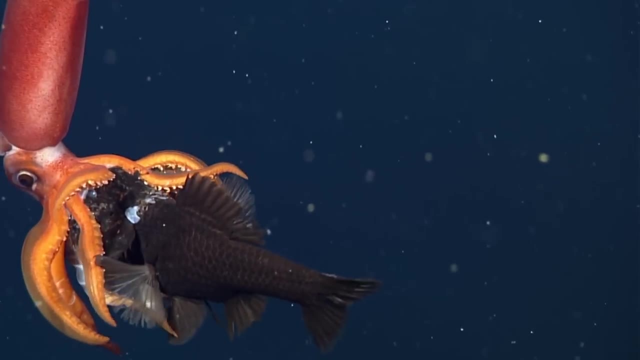 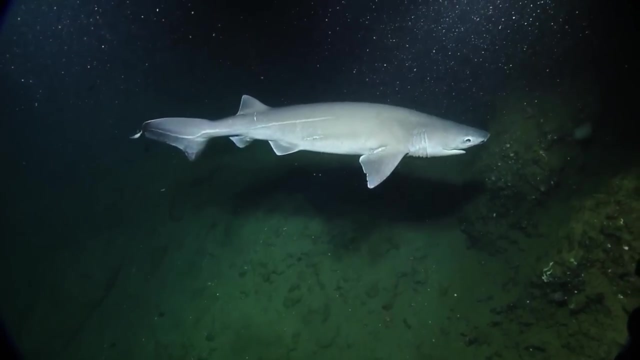 less abundant so far from the producers of the source. Pelagic wanderers can go for very long periods of time without feeding. Their slowed metabolisms are a useful adaptation down here, where nutrients are scarce. Even so, wanderers cannot rely entirely on residual nutrients brought to them from vents. 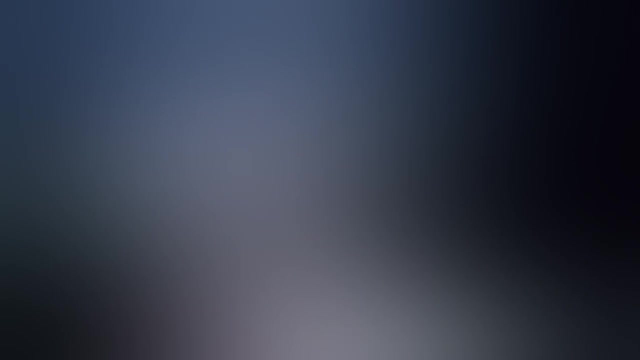 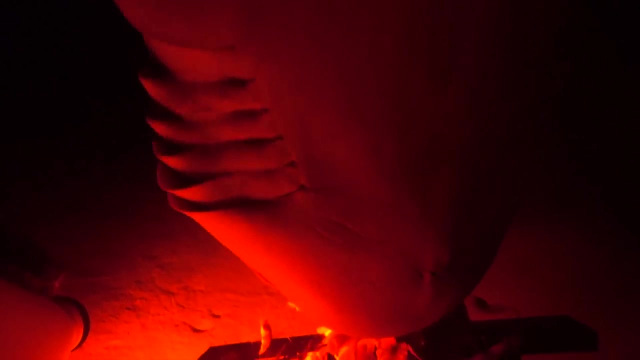 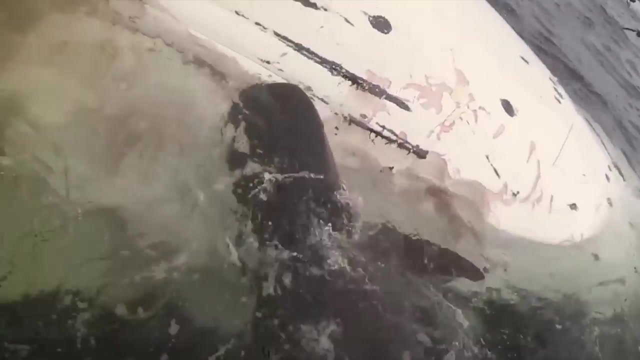 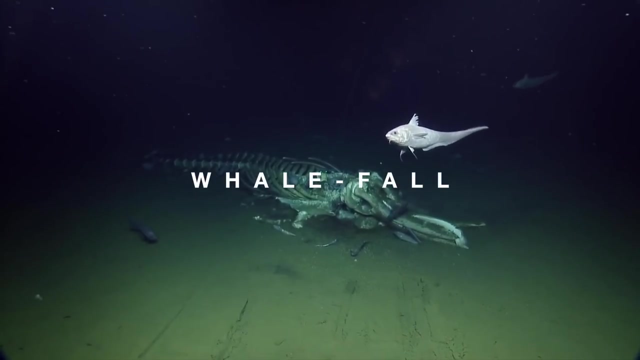 and seeps. They must become opportunistic feeders and be able to take advantage of any kind of food they come across Occasionally. amidst the constant trickle of marine snow from above, something larger will sink to the deep sea. This is a sunken whale carcass, known as a whale fall, that can support a complex biological 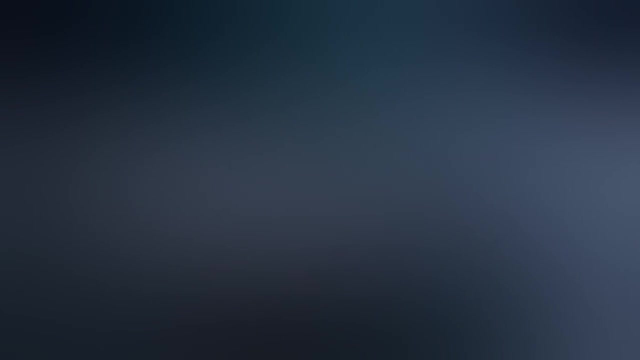 community for up to 50 years. This is a sunken whale carcass, known as a whale fall, that can support a complex biological community for up to 50 years. Within minutes of it reaching the sea floor, pelagic wanderers gather out of the barren. 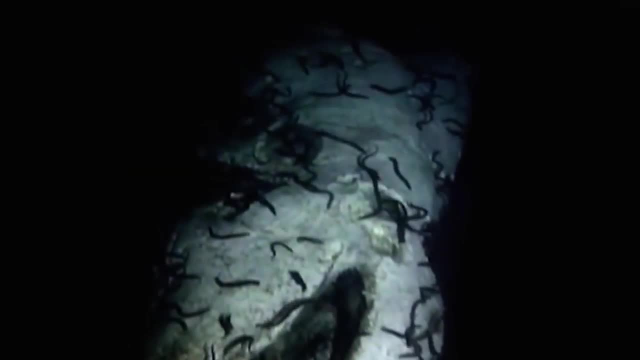 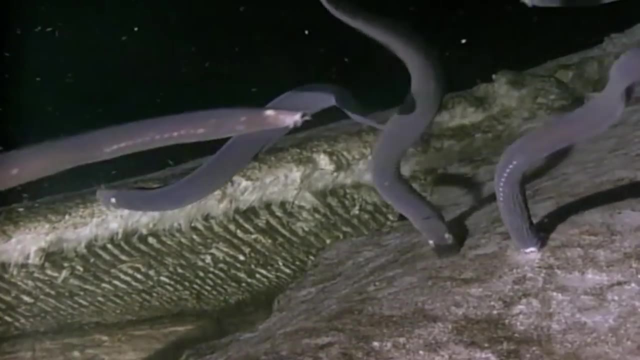 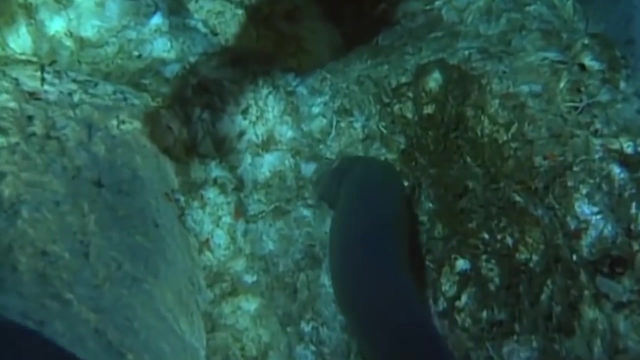 darkness to feed. The first to arrive are mobile scavengers. These are the larger ocean wanderers, including hagfishes and gigantic sleeper sharks, who take on the role of detrivores breaking down the dead matter. Whale falls attract such an abundance of life because their nutrient content is equivalent. 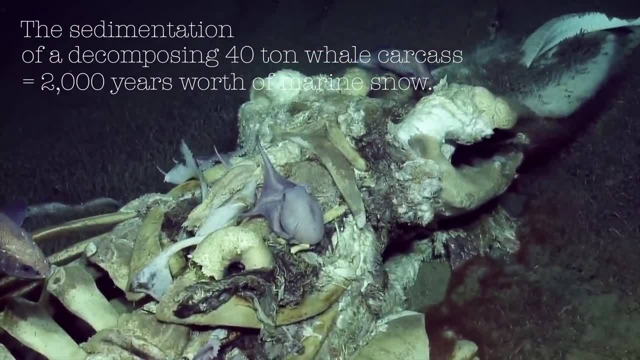 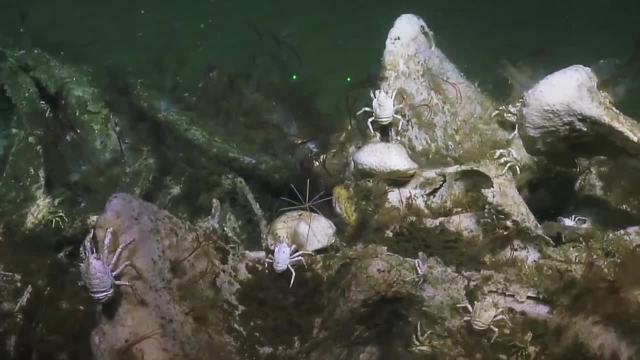 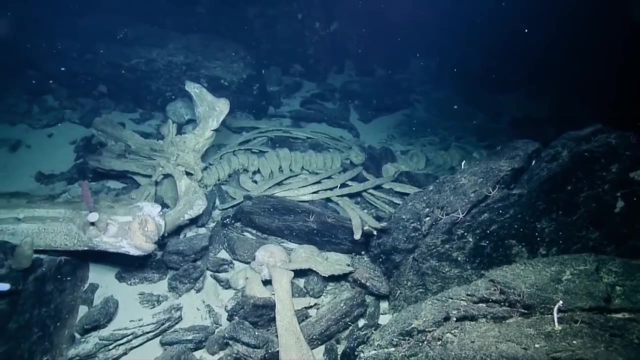 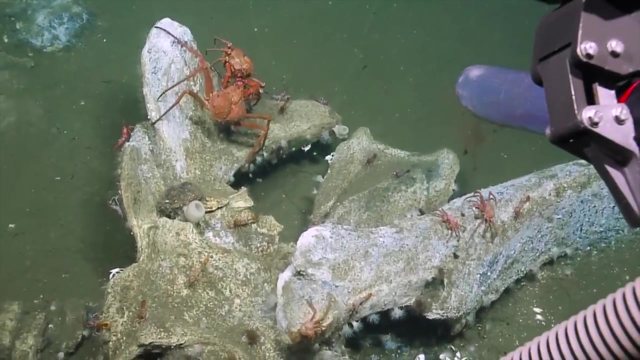 to 2,000 years' worth of marine snow, providing a rich supply of nutrients concentrated in one small area. Even once the soft tissue has been stripped, the remaining bones and scraps do not go to waste. During the Sulfophyllic stage of the whale fall ecosystem, the most important part of 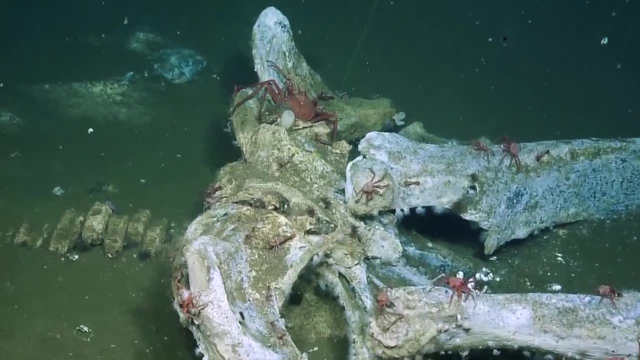 the ecosystem is the soil. The soil is the most important part of the ecosystem. It is the most important part of the ecosystem. It is the most important part of the ecosystem. It is the most important part of the ecosystem: The soil. it is the most important part of the ecosystem. 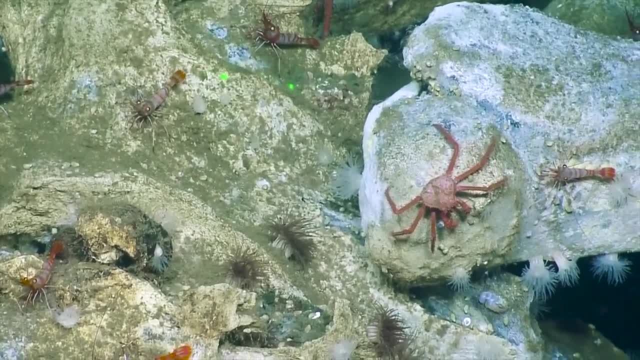 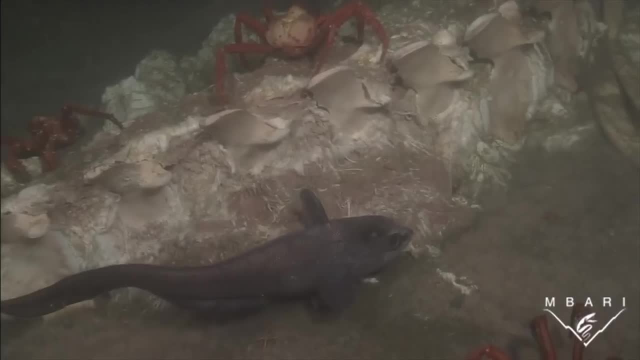 The soil is the most important part of the ecosystem. They have a very important role to play in the evolution of the biosystem. Chemosynthesis occurs here too, during which specialised bacteria break down the lipids present in the bones to produce sulphides. 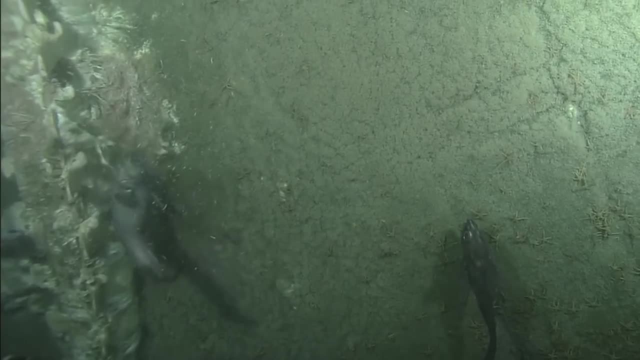 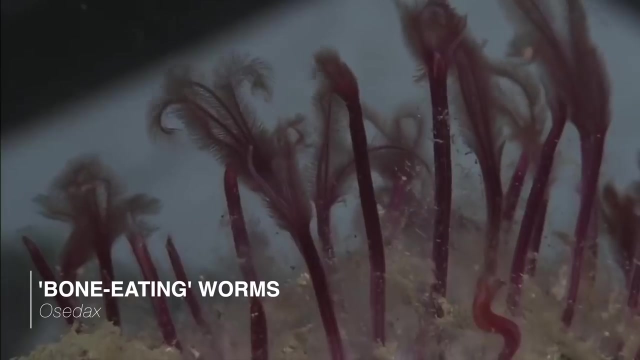 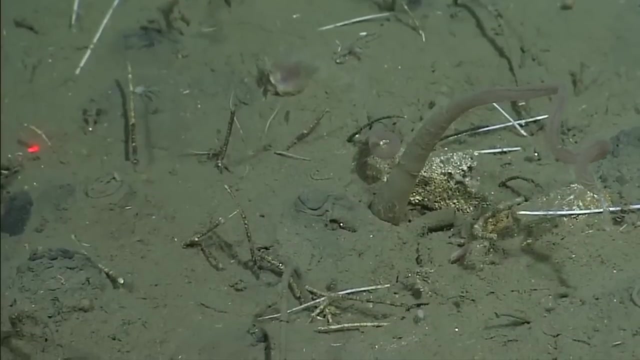 The presence of sulphides allows other organisms to thrive, including dense mats of bacteria, mussels and tube-worms. But unlike hydrothermal vents, whale falls are temporary. They have to be interminablyhybridated, cannot specialise to rely on them for nutrients. There is simply not enough time to allow creatures. 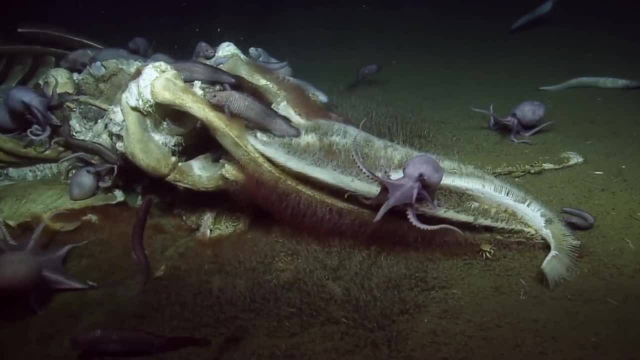 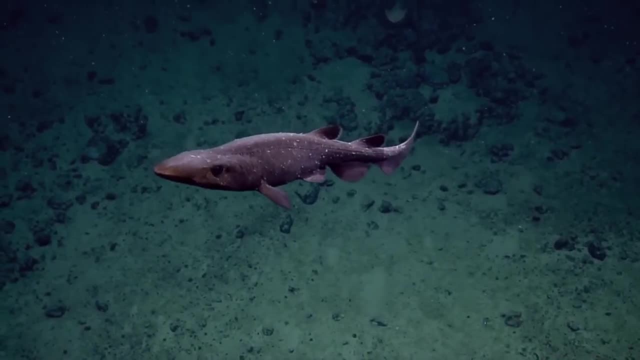 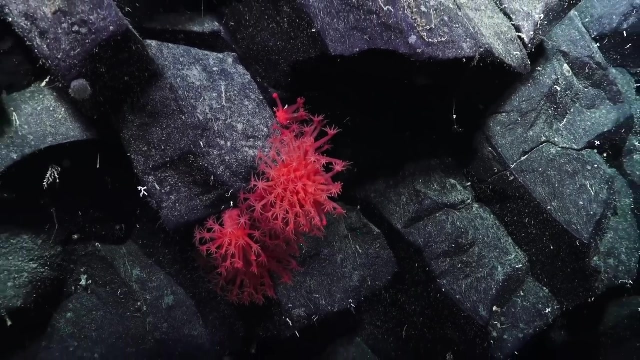 to evolve here. so these sunken carrion remain to be transient feasts for the pelagic wanderers who, once the flesh has been stripped, dissipate once more into the barren expanse in search of prey. Overall, these isolated ecosystems in the deep sea are all interconnected With 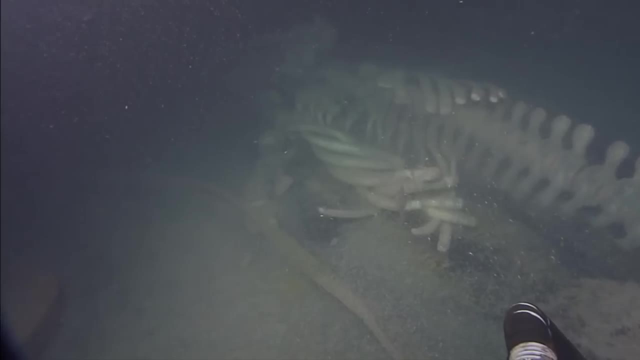 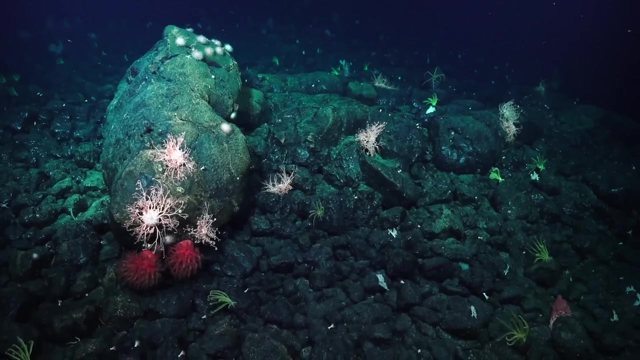 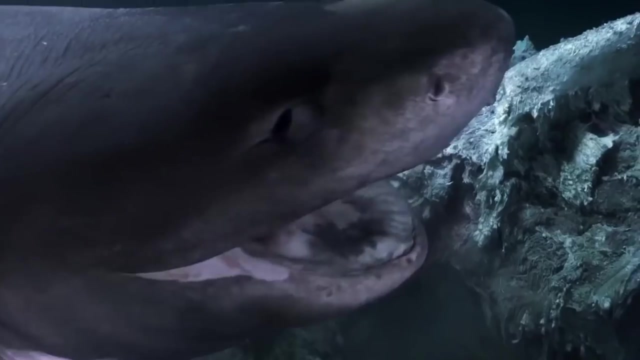 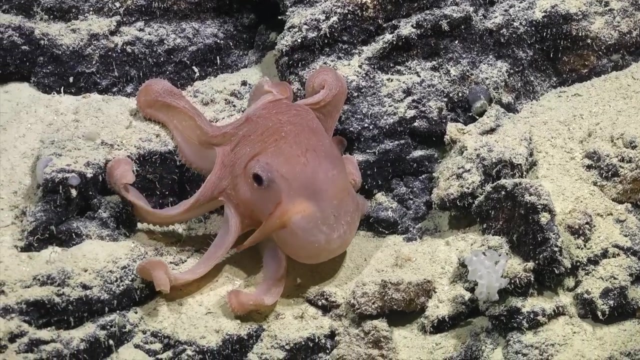 each one relying on the processes of energy production, predation and decay to transport nutrients between communities. The depths benefit from productivity in the shallows, supporting filter-feeding detritivores that in turn, support predators. Due to the loss of energy between trophic levels, predators display unique adaptations to make them more. 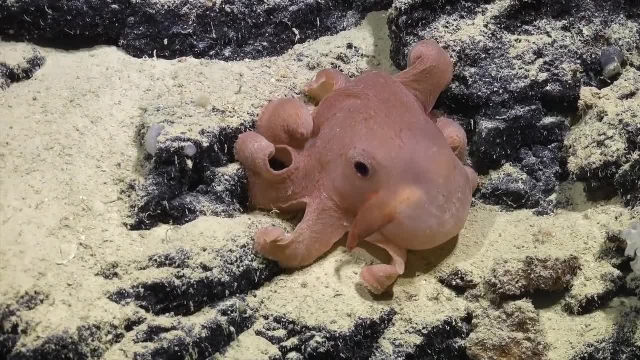 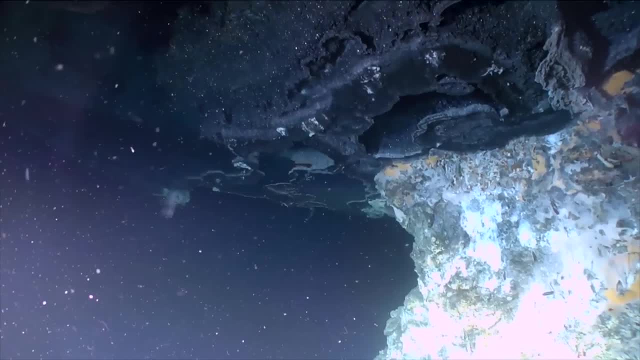 efficient Nutrients flow between the isolated ecosystems. Taken from the soil, they are then transferred to the surface of the sea and then to the deep sea through hydrothermal vents, out into the open ocean, where they are cycled further through death, decay and defecation. Thus, the habitats and inhabitants of the